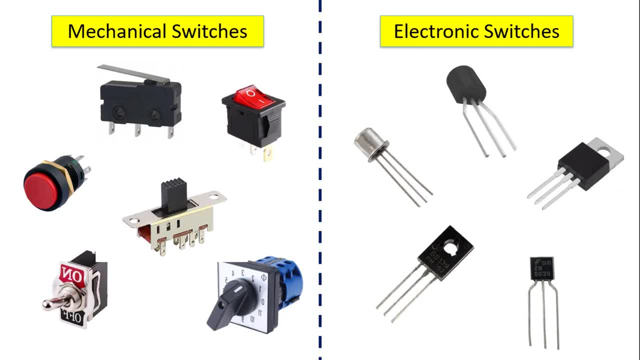 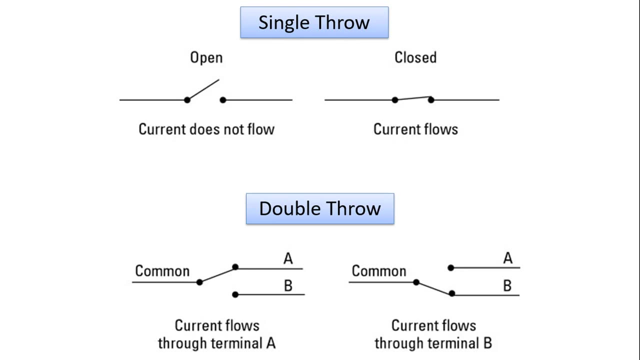 switch is activated differently and does not need physical contact. Instead, it is activated by semiconductors such as transistors. This lesson will focus on mechanical style switches. Many mechanical style switches are categorized by their number of poles, throws and style of. 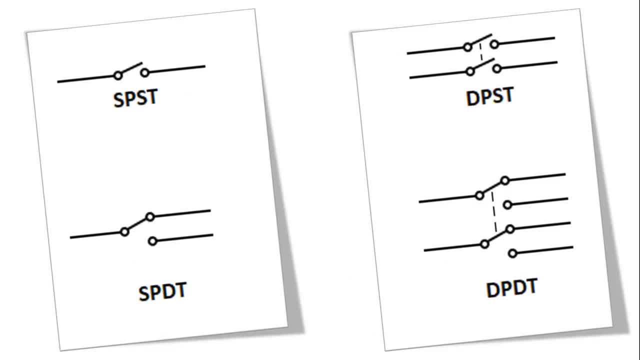 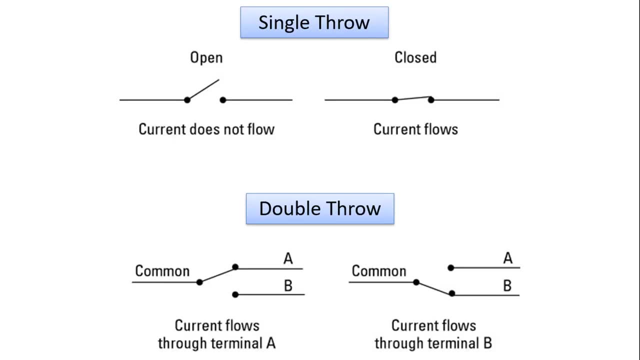 up and down. This is an example of a mechanical switch and a mechanical switch, A mechanical operation. Polls and throws are simply denoted by letters spst, spdt, dpdt, for example. To better understand the working logic of switches, we need to know the concepts of. 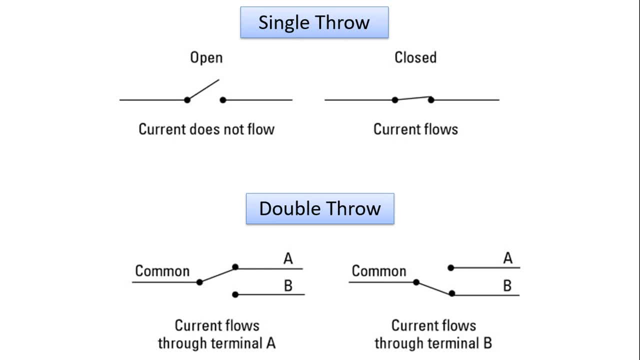 polls and throws. Polls tell you how many separate circuits a switch can control. A switch with one poll can direct one circuit, Two polls can direct two circuits, and so on. How many positions can be activated by the switch. A single throw can close a circuit at one position, whereas a double throw switch can. 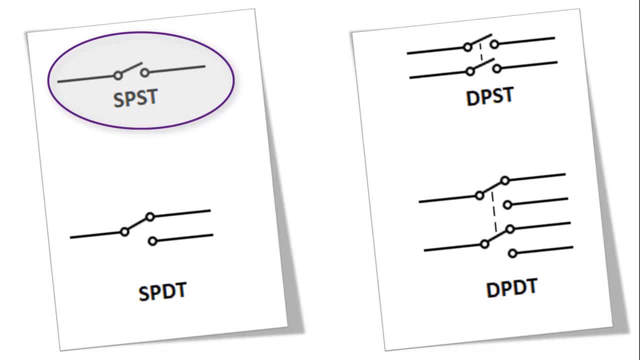 close a circuit in two positions. An spst or single poll, single throw switch is the simplest form of mechanical switch. It is a simple on-off switch with one input contact and one output contact. It switches a single circuit and can either make or on or break or off. 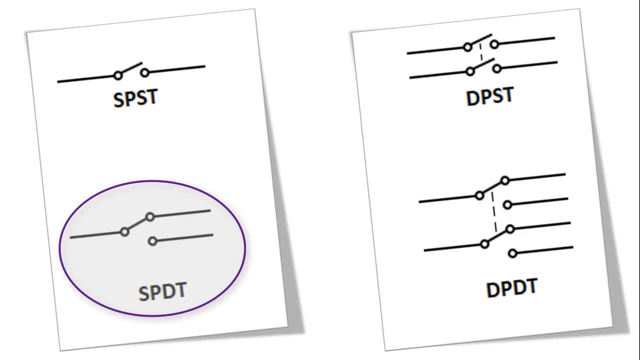 An spdt or single poll, double throw switch has three terminals, one more than the simple spst switch. It has one input contact and two output contacts. This means that an spdt switch has two on positions and one off position. 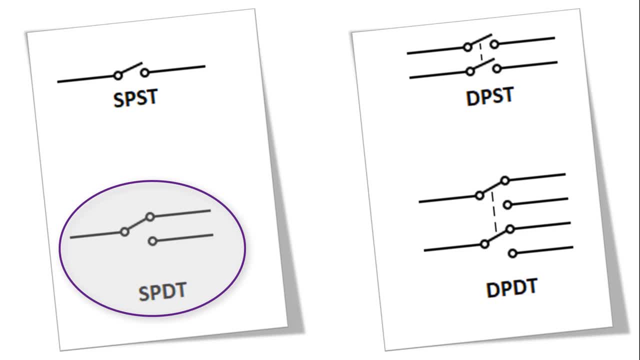 Most slide switches have an spdt configuration and are used to change over between two outputs. A dpdt or double poll double throw switch has six terminals. It is simply two on-off positions. It has two spdt switches. The switch has two input contacts and four output contacts, commonly used as on-on or 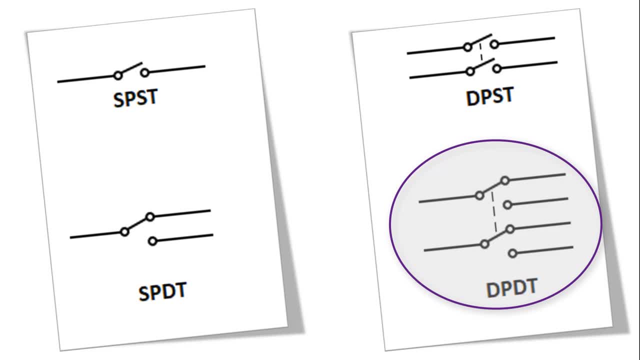 on-off on switches. A good visual example for a dpdt switch is controlling car turning indicators. Activating the switch up would turn on both the front and back car indicator in one direction. Activating the switch down would turn on both the front and back indicators in the opposite. 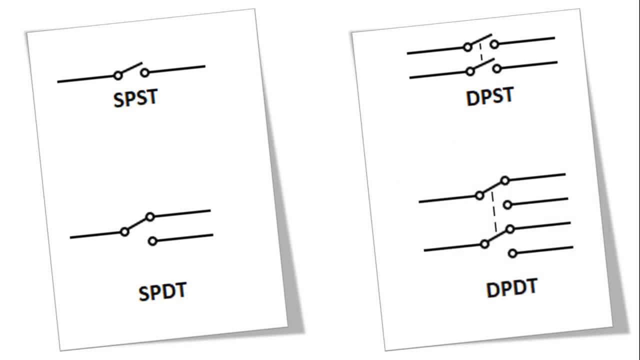 direction. A momentary double poll, double throw switch requires the switch to be pressed or held continuously for the operation to work. When it is released, the switch will stop. For example, the switch is on your keyboard. When they are released, they no longer operate. 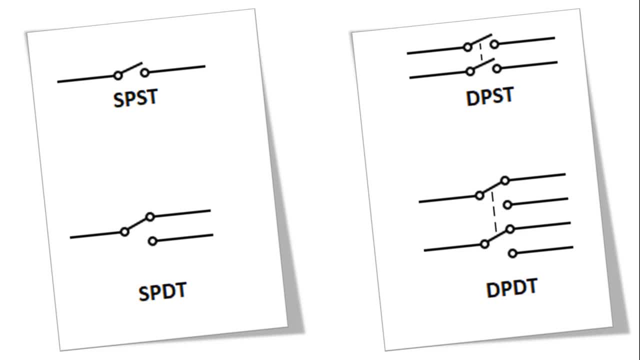 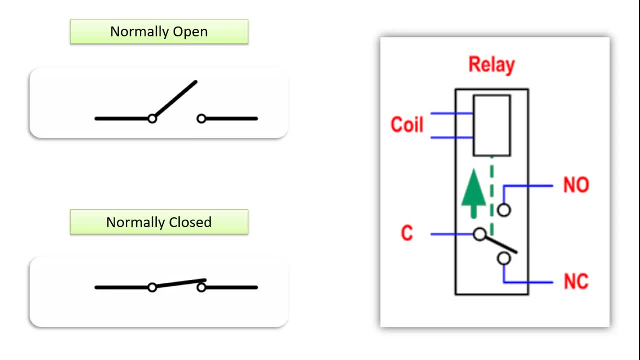 A latching switch will stay on or off until it is pressed again, For example a light switch. Now let's examine the concepts of normally open or NO and normally closed or NC. Simply, a closed switch allows current flow and is therefore on. 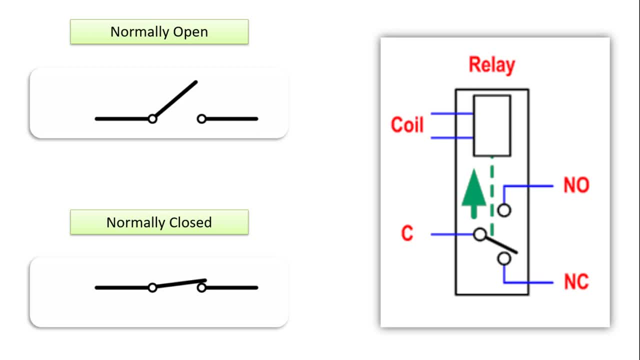 An open switch does not allow current flow and is therefore off. A normally open, NO switch has an off resting position. When the switch is pressed, it becomes a closed circuit and is therefore on. A normally closed switch has an on resting position. When the switch is pressed, it becomes an open circuit and is therefore off. 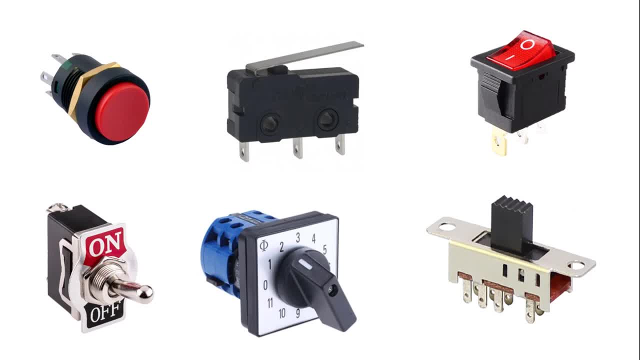 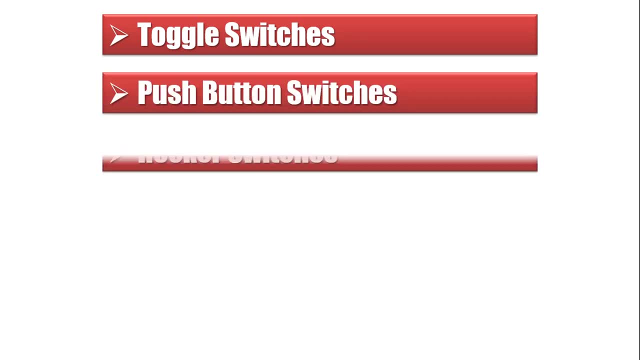 Now let's examine the types of mechanical switches. This section we will look at the most common types of mechanical switches. These are toggle switches, pushbutton switches, rocker switches, rotary switches, slide switches and micro switches, to name a few. 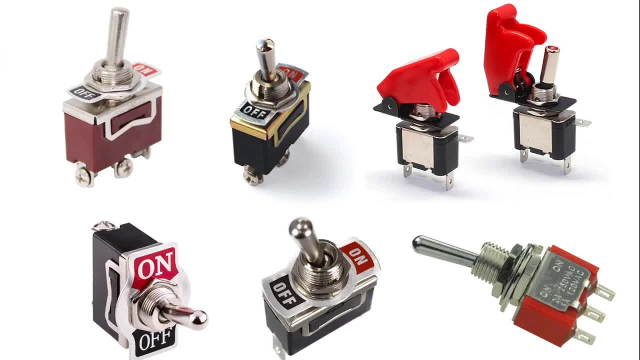 Number 1. Toggle switches. A toggle switch is a type of electrical switch that is actuated by moving a lever back and forth to open or close an electrical circuit. There are two basic types: maintained contact and momentary toggle switches. A maintained switch changes its position when actuated and will remain in that position. 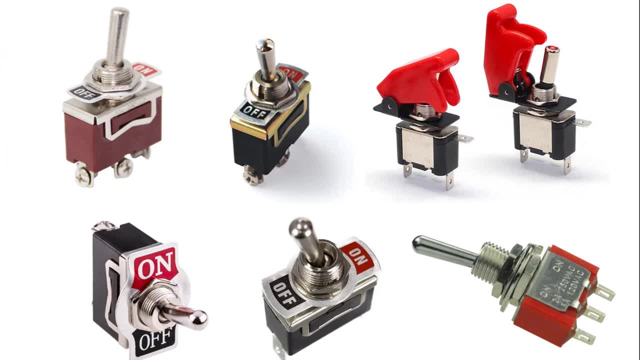 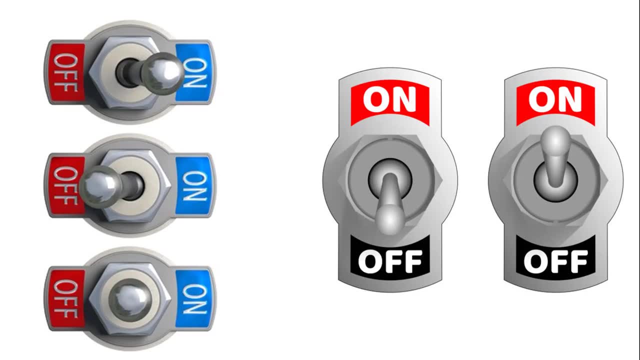 until actuated again, such as an on-off function. A momentary toggle switch is actuated only when someone is operating the switch. A toggle switch is actuated by a lever that can be flicked into one, two or more positions to actuate the switch, most commonly described using the pull and throw. 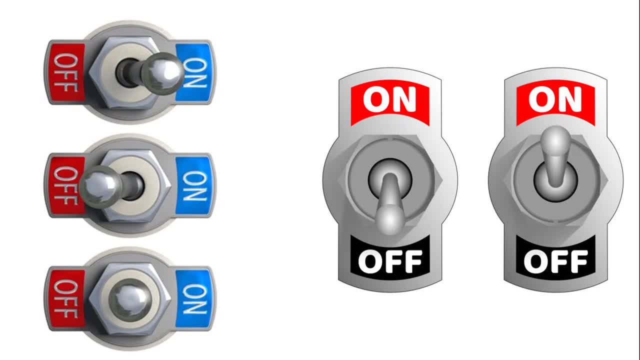 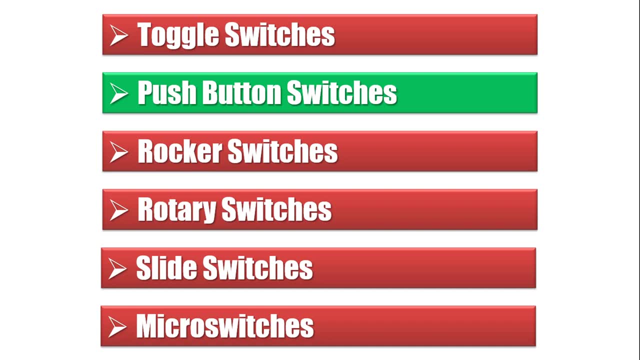 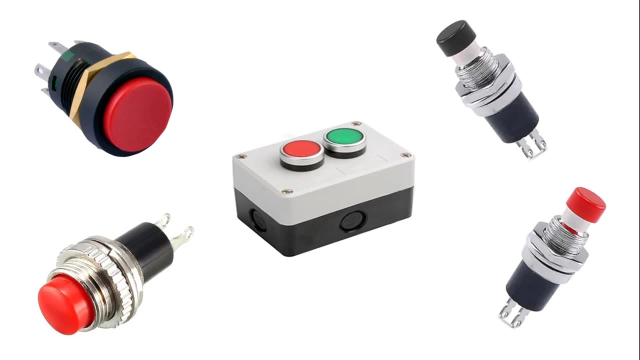 notation described in the previous section. A momentary toggle switch will spring back to the original position when pressure is released. Number two: push-button switches. A push-button switch causes a temporary change in an electrical circuit only. while the switch is physically pushed, A spring returns the switch to its original position immediately afterwards. The 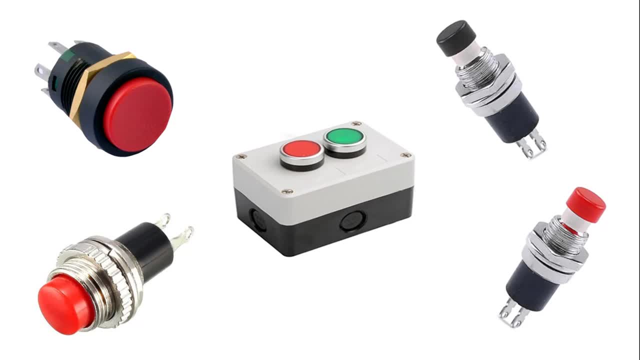 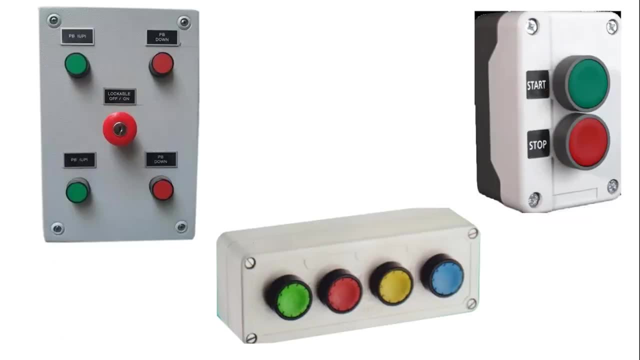 push-button is typically made of plastic or metal and may be flat-surfaced or contoured to the finger or hand. also known as momentary switches, The most common type of two-position switch, come in a variety of shapes, Styles and materials. Pushing the button will either make on or break off a circuit. The 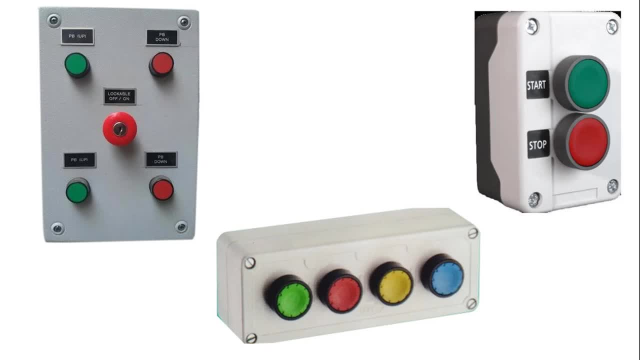 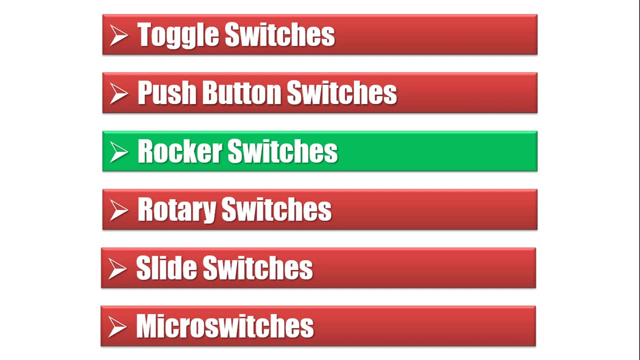 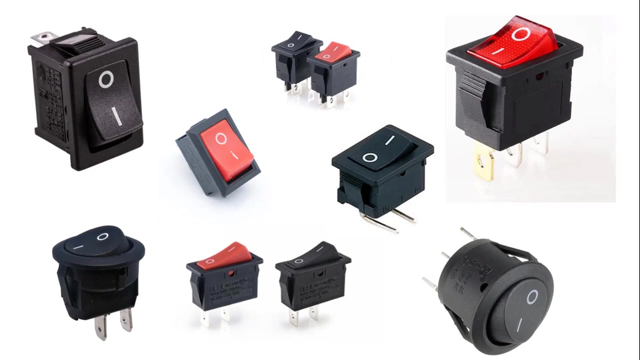 action can either be latching or momentary. A latching switch will stay on or off until it is pressed again. Number three: rocker switches. A rocker switch is an electrical switch that rocks back and forth and is actuated by a paddle- standard rocker or dual rocker- A rock switch. 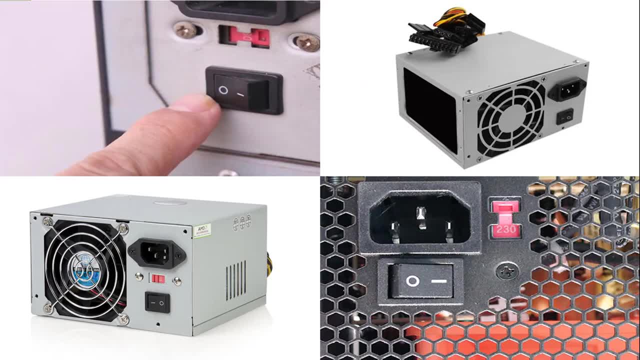 has a seesaw-type action whereby pressing one switch will make a rocker switch. A rocker switch on one side will rock the button in that direction and close the contacts on. Rocking the switch back to the alternate slide will open the contacts off. Many styles and shapes are available in. 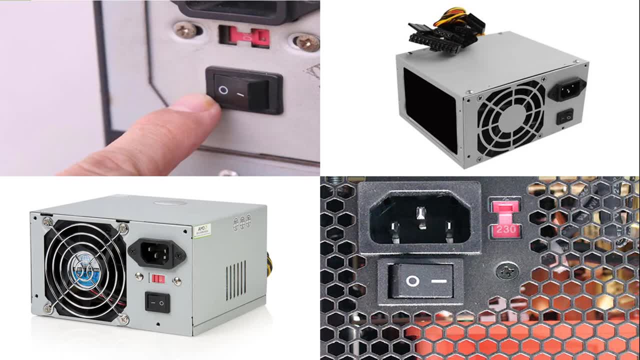 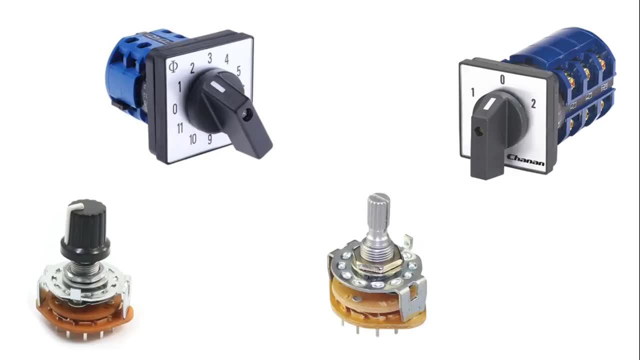 single-pole and double-pole configurations. for example, Number four, rotary switches. Rotary switches move in a circle and can stop in several positions. A rotary switch is used to control many electrical circuits with a single switch and can be designed to have many contacts. 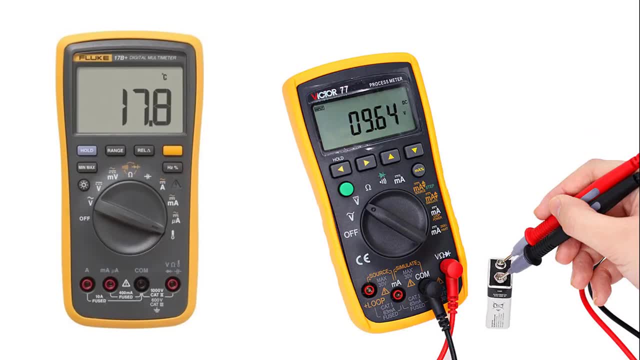 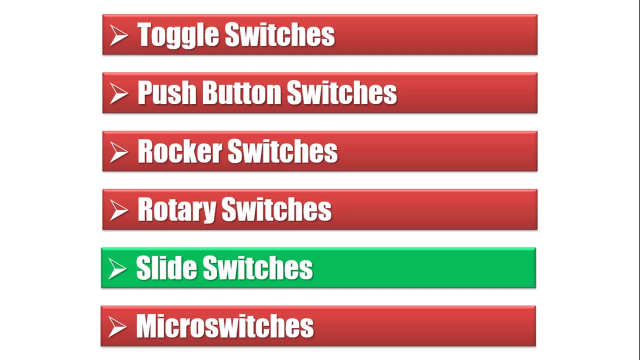 at once on a single switch position. A rotary switch is turned in order to open or close the contacts of the switch. It consists of a moving contact which is turned in order to connect with the stationary contacts. A visual example would be the dial on a cooker Number five slide switches. 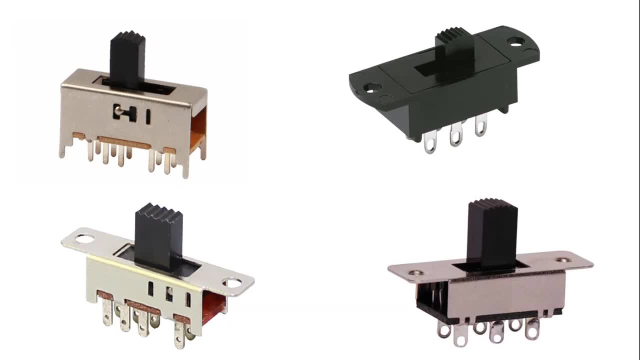 Commonly have a small knob that can slide in order to open or close the switch contacts. They are very compact and easy to operate, making them ideal for small-scale projects or circuits where changeovers are required, for example within model railways. 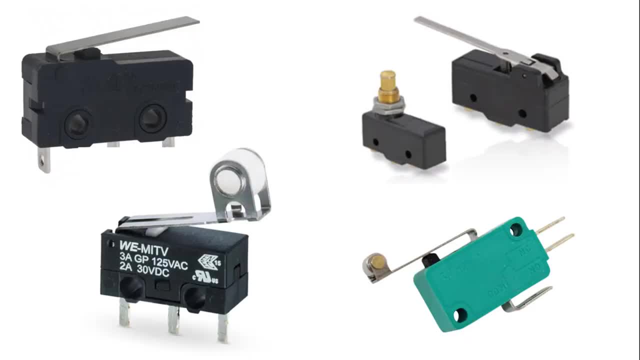 Number six: microswitches. Microswitches have either a small push button or a lever in order to actuate the switch. They require very little physical force in order to operate and are ideal for small-scale projects or applications. They use a tipping point mechanism sensitive to small. 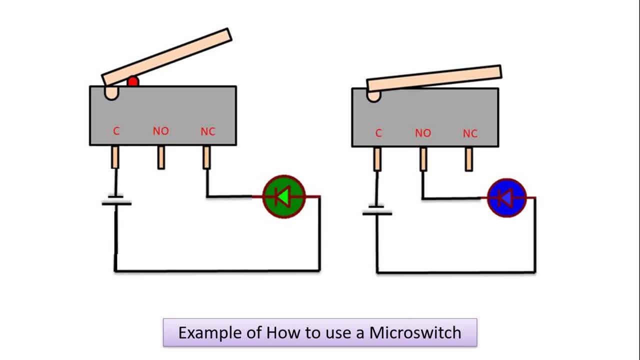 actions. A common practical example of a microswitch in action would be within a microwave door. If the door is opened whilst the microwave is operating, the switch lever is released and the contacts are open, stopping the machine. These are the types of mechanical switches that we can.